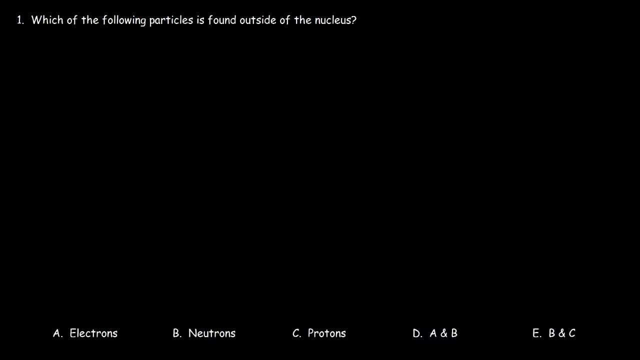 answer choices listed here. Well, let's talk about the structure of the atom. In the center of the atom, which is known as a nucleus, you have the protons, which I'm going to write in red, and the neutrons, which I'm going to put in brown. 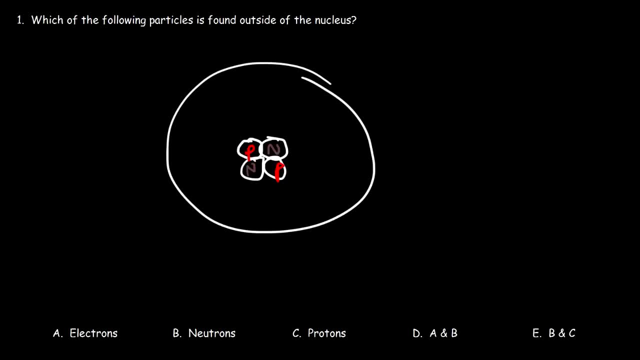 Outside of the nucleus are the electrons. The electrons are orbiting the nucleus, and so the electrons form the electron cloud, but the nucleus consists of the protons and the neutrons. Now the atom is mostly empty space, Even though this picture doesn't show it to scale. 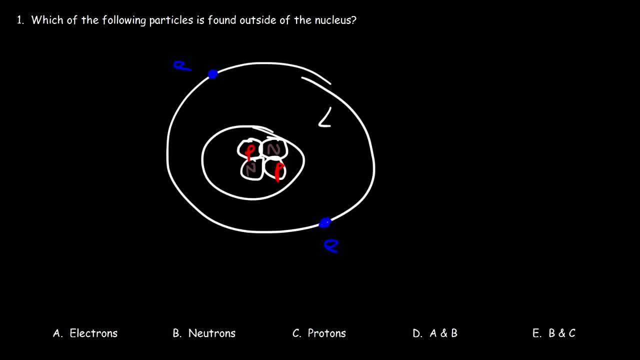 this nucleus is relatively small to the electron cloud, and so a lot of matter like high-energy particles can go straight through an atom. because an atom is mostly empty space, 99% of the mass is concentrated in the nucleus of the atom. Protons and neutrons are almost more than 1,800 times more massive than 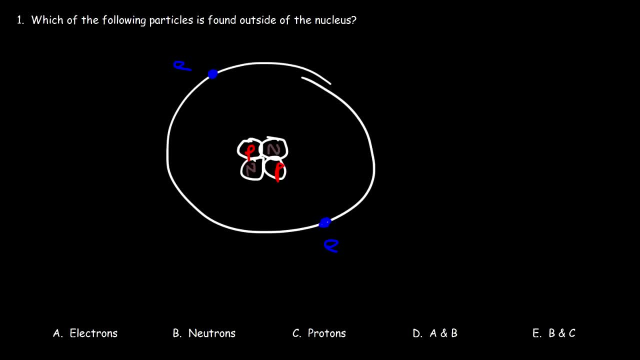 an electron. So, going back to this question, the particles that are found outside of the nucleus are the electrons. A is the right answer to this problem. Now let's move on to this problem number two: Which of the following subatomic particles carries a positive charge? Is it the electrons, the neutrons or the? 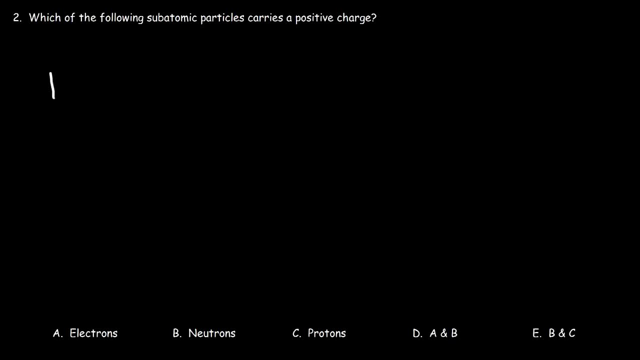 protons, Neutrons, are electrically neutral. They don't have a charge. Think of N for neutral. Protons carry a positive charge, Think of P for positive, And electrons carry a negative charge. but you have to just know that by. 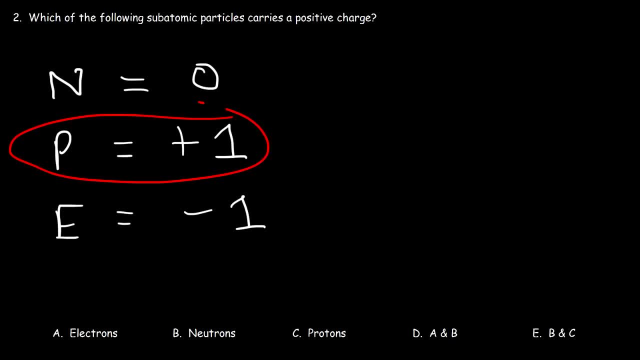 elimination. So the answer for this one are the protons. They carry the positive charge, So C is the right answer. Now, going back to the structure of the atom, I have some questions for you. So we said that at the center we have the protons which carry a positive charge. 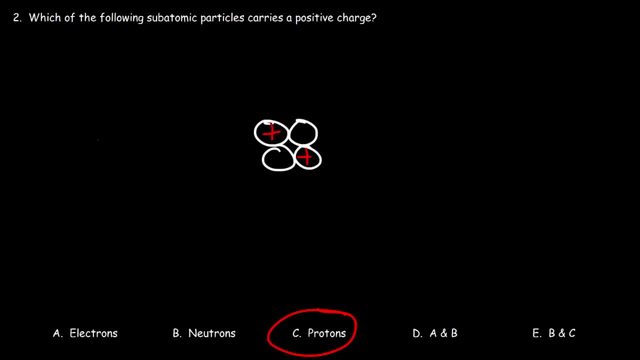 and the neutrons, which carry a neutral charge or no charge at all, and the electrons which orbit it, and they carry a negative charge. Now, perhaps you've taken physics and you know that opposite charges attract. So if you have a 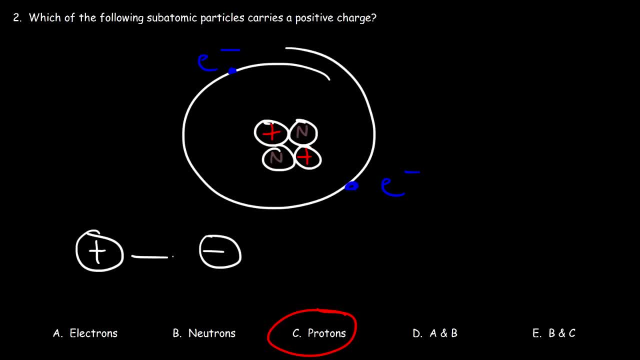 positive charge and a negative charge, there is an electrostatic force of attraction That accelerates them toward each other. So therefore the electrons are attracted to the nucleus. So why don't the electrons just fall into the nucleus? What keeps them in orbit around the nucleus? It turns out that their speed keeps them in. orbit, They're moving pretty fast Whenever you have an object that's moving in one direction and if there's a force that's perpendicular to the motion of the object, the force doesn't change the speed of the object. Rather, it changes the direction. 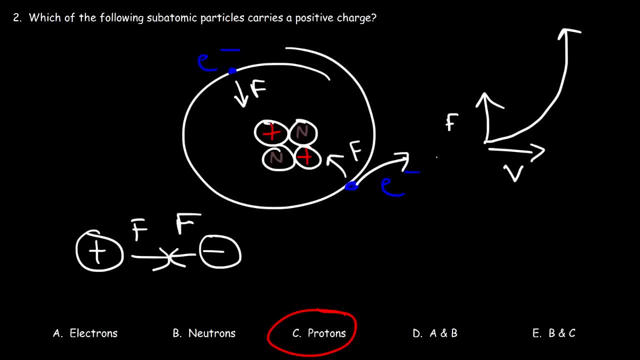 of the object. So the electron at this point wants to fly outside of the atom. but the electrostatic force between electrons and protons help keep it in orbit. So the electron doesn't fly out of the atom or doesn't really fall into the nucleus, As long as it maintains the right energy. 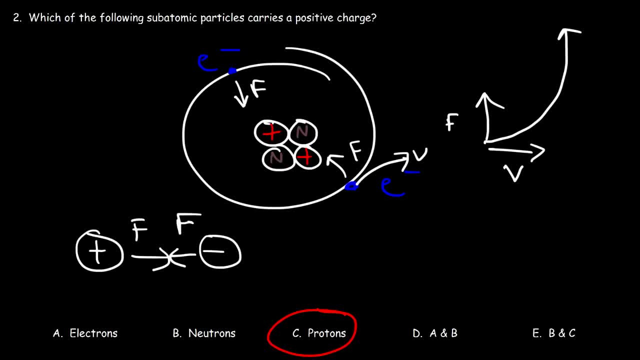 Now, if the electron absorbs a photon and gets a lot of energy- sometimes it's kinetic energy might be high enough where it can fly off and leave an atom if it has the right energy. And there are times where an electron actually can fall in the nucleus and a nuclear reaction can occur. but that's a whole. 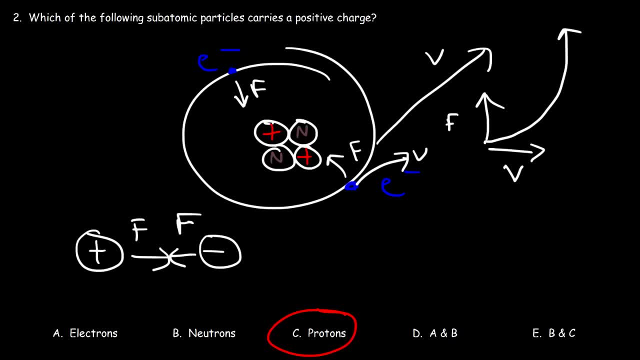 another topic, But for the most part electrons tend to stay in their orbit. The combination of the electrostatic force and their tangential velocity keeps them in orbit. Now, when the electron does fall into the nucleus, that process is known as electron capture. You can actually look it up. And when that 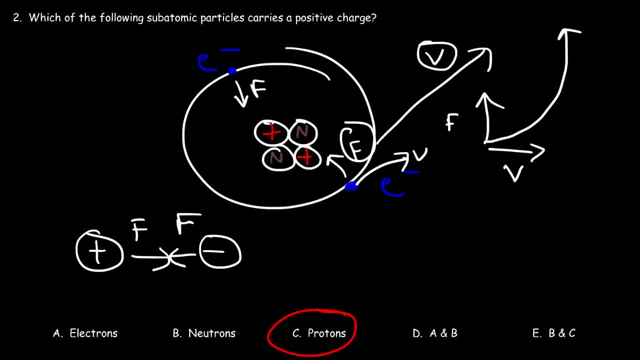 happens, the chemical identity of the substance actually changes. The element changes from one element to another, And so the electron sometimes can fall into nucleus, and other times, if it gains a lot of energy, it could fly away from the atom, turning into an ion, And an ion is. 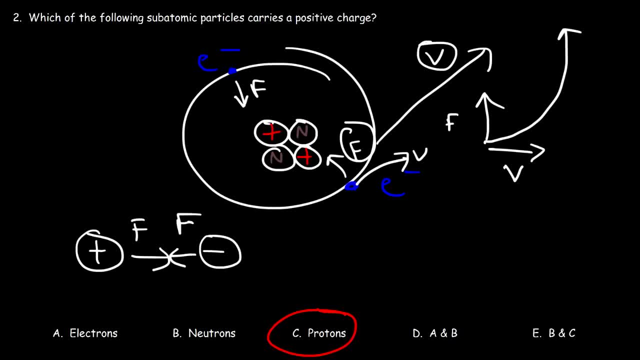 basically an atom that can fall into a nucleus and other times, if it gains a lot of energy, it could fly away from the atom, turning into an ion, And an ion is basically a particle with unequal numbers of electrons and protons, But these things are not the norm. 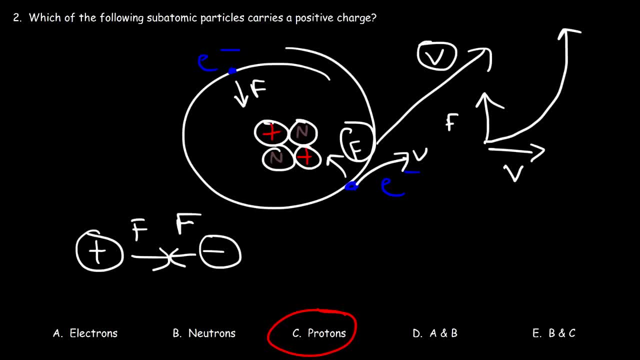 For the most part, an atom is electrically neutral, understanding conditions and electrons tend to maintain in their orbits, So they don't always just leave just like that. Now here's another question for you. If like charges- I mean if opposite charges- attract, then that means that like charges. 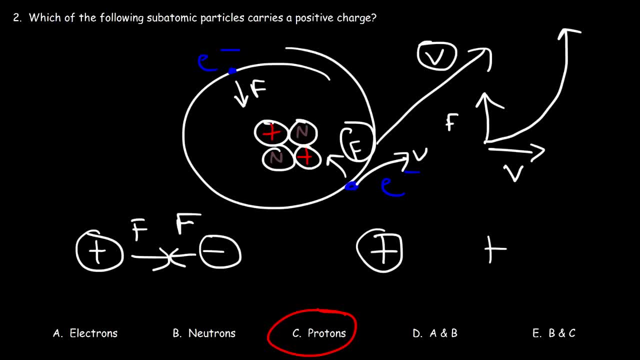 must repel each other. So if we put two protons next to each other, they should feel a force that will accelerate them away from each other. Inside a nucleus, you have two protons that are very, very close to each other. 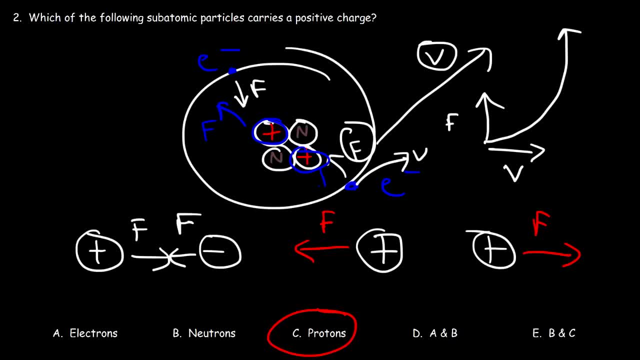 So, therefore, the electrostatic force has a tendency to pull them apart. So what keeps the nucleus together? What keeps the protons so close to each other, when we know that, like charges, they repel? And it turns out there's another type of force within the nucleus of an atom? 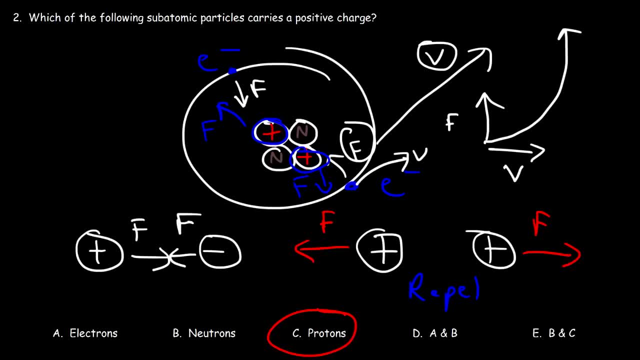 It's known as the strong nuclear force. It's very powerful, much stronger than electrostatic force, And it keeps the nucleus together. It prevents the protons from flying apart And, as you've seen, nuclear reactions are far more powerful than chemical reactions. 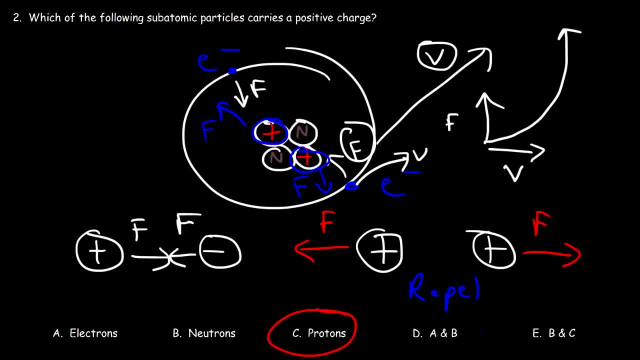 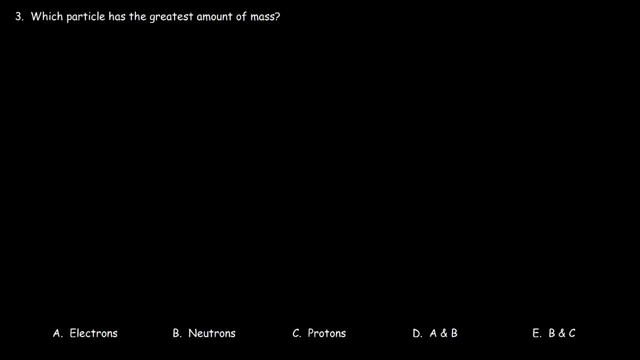 The strong nuclear force. it's a lot stronger than electrostatic force. Number three: which particle has the greatest amount of mass? The mass of a proton is 1.6726 times 10 to the negative 27 kilograms. It's very, very small. 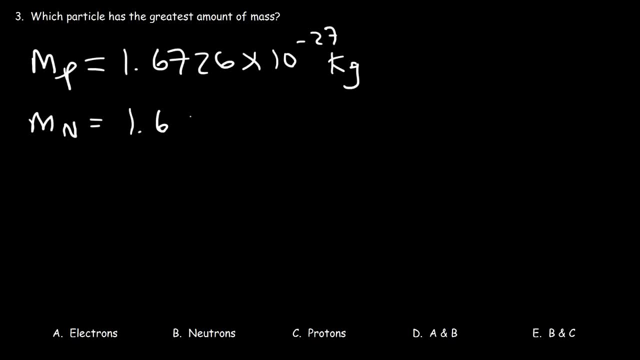 And the mass of a neutron is 1.6749 times 10 to the minus 27.. So a neutron is slightly heavier than a proton. Now the mass of an electron is a lot smaller. It's 9.11 times 10 to the minus 31.. 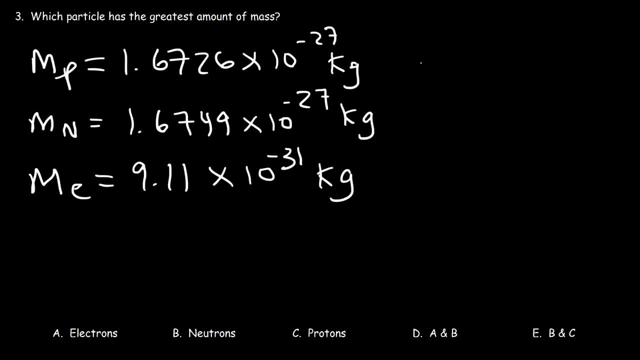 Now you might be wondering: what do these numbers mean In terms of atomic mass units, a proton is approximately one atomic mass unit. The same is true for a neutron. Now, a neutron is slightly more heavy than a proton, But in terms of atomic mass units, 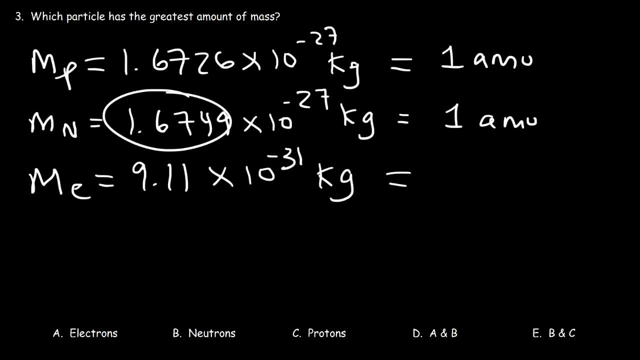 these two are very close to each other and they're approximately one. The electron is a lot lighter than the proton or the neutron, And it's about 0.000549 atomic mass units. So the atomic mass of an element is based on the number of protons and neutrons. 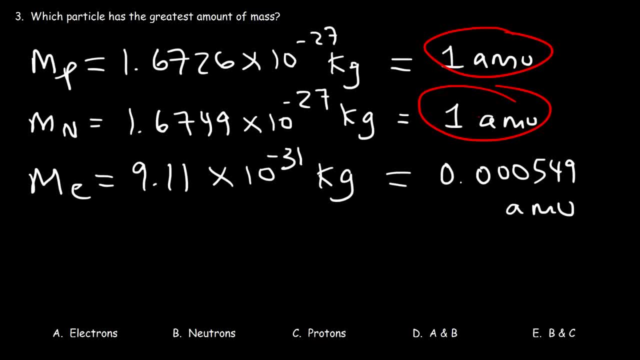 Because the electron is so light relative to a neutron and a proton, the mass of the electrons within an atom, the mass of the electrons within an atom, is considered to be negligible, So the particle with the greatest amount of mass in this problem is the neutron. 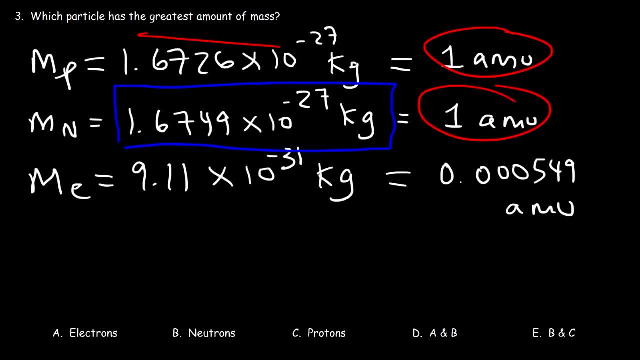 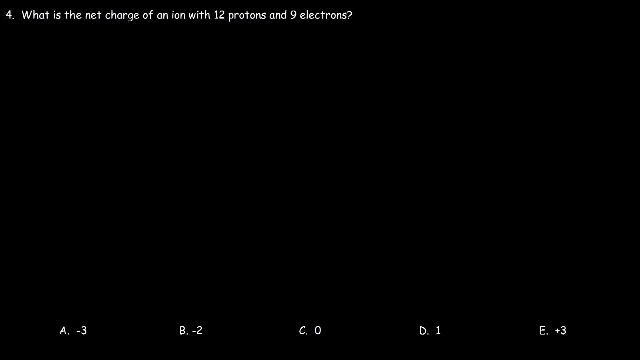 It's slightly more heavier than a proton Number four. What is the net charge of an ion with 12 protons and 9 electrons? To calculate the net charge, it's simply equal to the sum of the charges of the protons and the electrons. 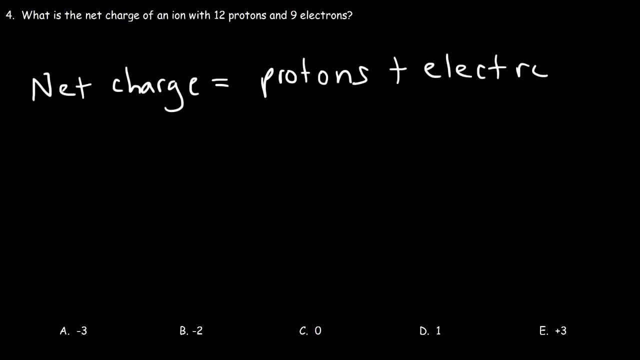 Just keep in mind: a proton bears a positive charge and an electron bears a negative charge, So we have 12 protons each with a charge of plus one. So it's going to be plus 12,, since there are 12 protons. 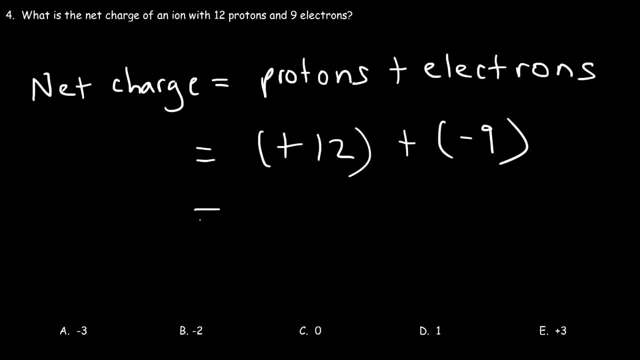 And we have nine electrons, so it's going to be plus negative nine. Therefore, the net charge of this ion is going to be positive three. It has a positive charge because there's more protons than electrons. If it has more electrons, it would have a negative charge. 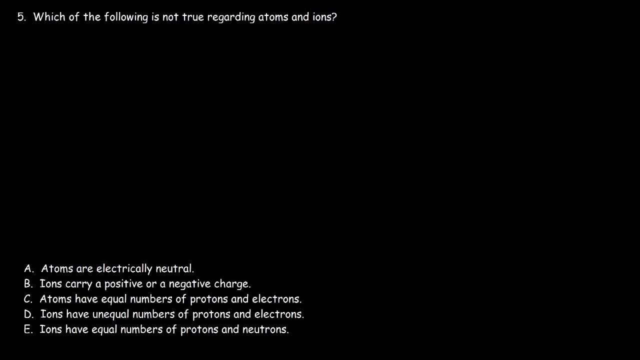 And so the answer for this one is E, Number five. Which of the following is not true regarding atoms and ions? So let's look at A. Atoms are electrically neutral. Is that true? It turns out it is, So here's an example. 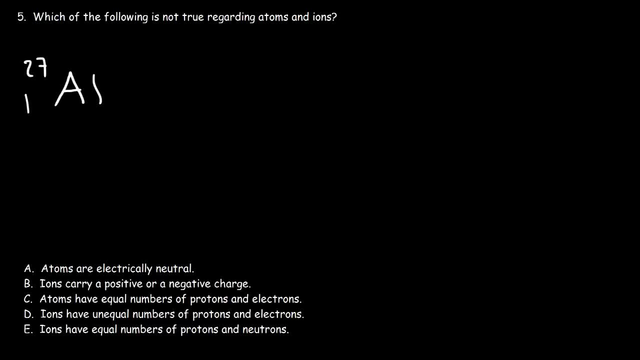 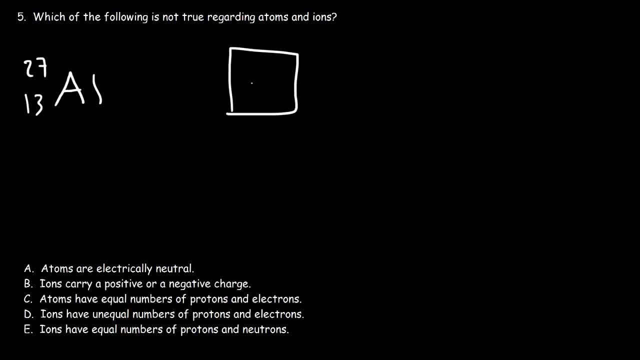 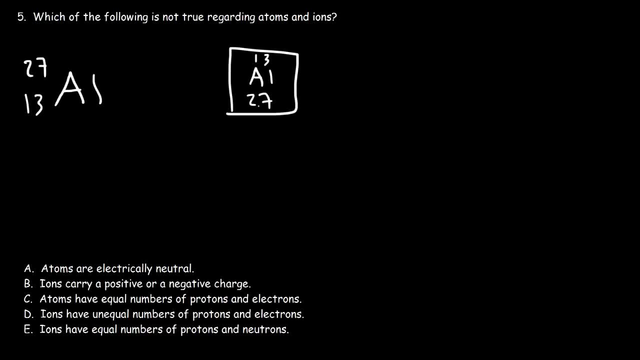 It might have a 13 on top and a 26.98 on the bottom, which I'm going to round to 27.. The larger of the two numbers is always the mass number, The smaller one is the atomic number. Now, the number of protons is always equal to the atomic number, which is 13.. 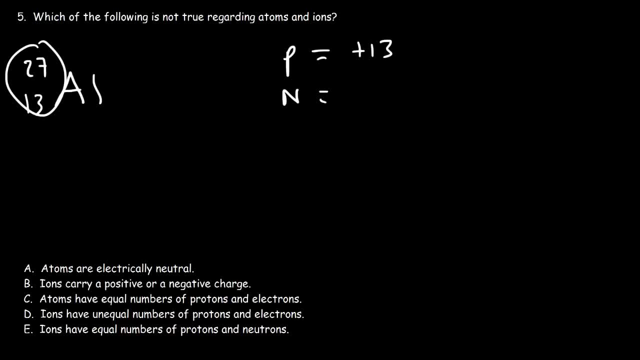 The number of neutrons is the difference between the mass number and the atomic number, So 27 minus 13 is 14.. The number of electrons is equal to the atomic number, which is 13 minus the charge. So there's no charge in this case.